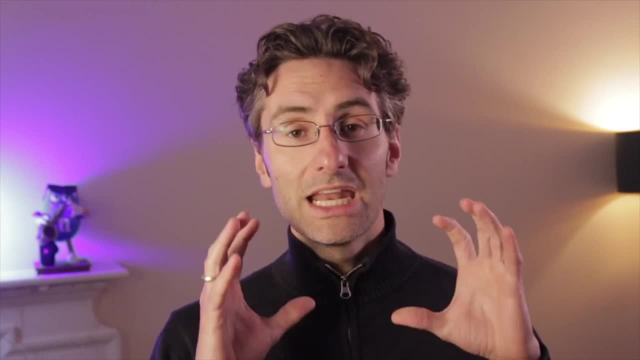 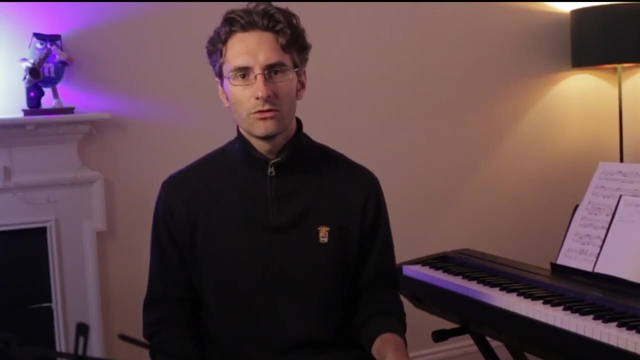 notes and how to play them. Let's get started. Let's start with quarter notes. I want you to do this with me. Just copy exactly what I do. It's not really hard, right? You're just tapping your hand on your leg, That's all Okay. 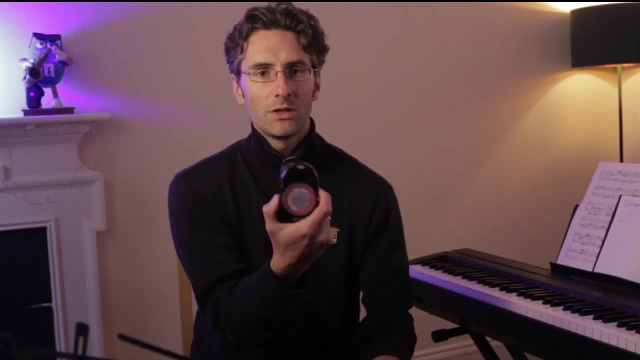 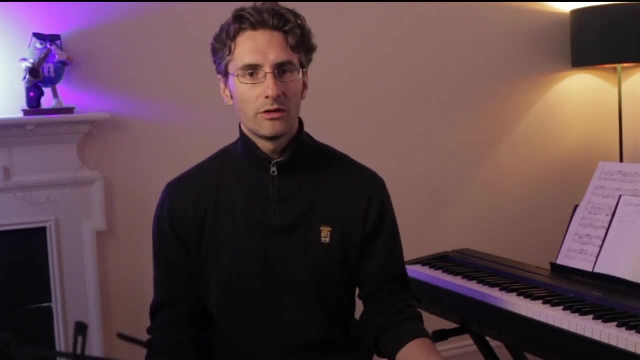 so that's fine. Now, if we get our metronome and we put the metronome at 60 BPM, okay, we're just going to tap along with the metronome, Not a big deal. One, two, three and four. 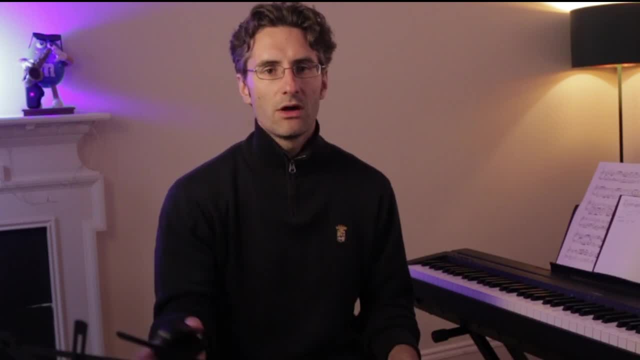 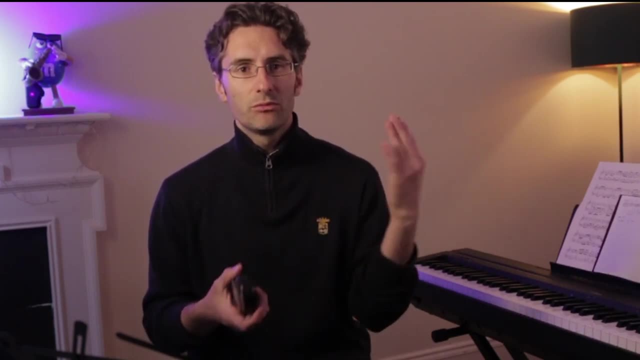 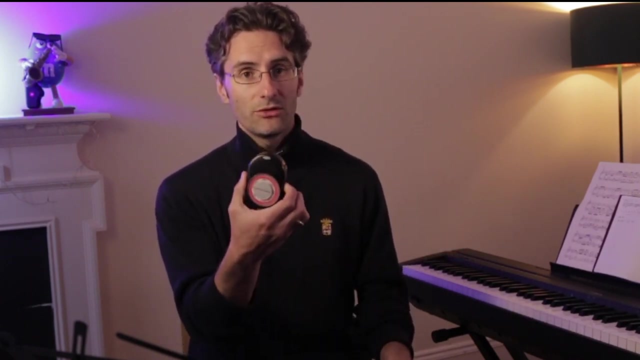 Two, three, four, Okay, now 60 BPM. the metronome is giving us the pulse, the heartbeat, Okay, and it happens that we're also playing the quarter notes, which correspond to the beat. So the quarter note and the metronome are in sync. They're exactly the same thing in this case, Okay. 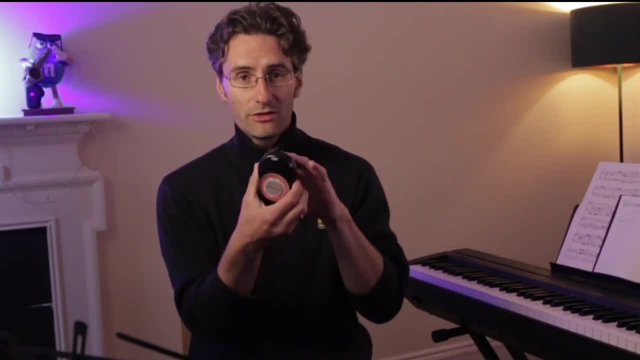 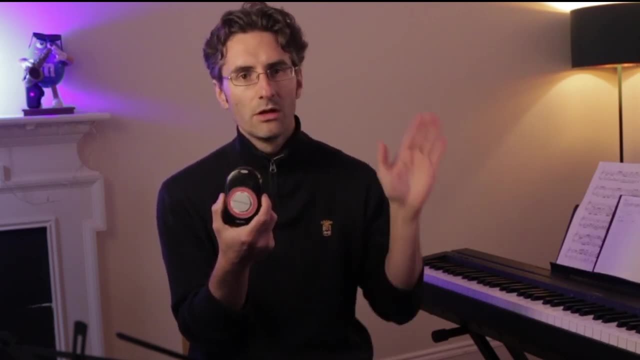 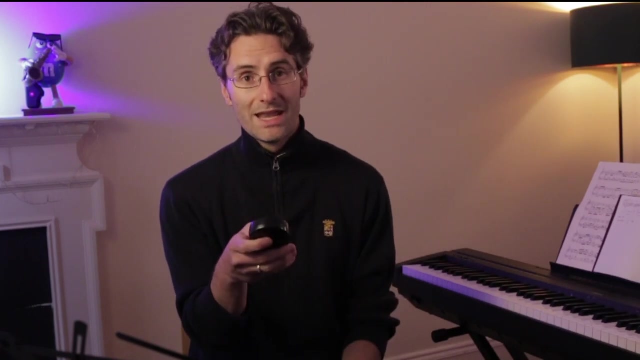 different note values afterwards, Okay, but in this case this and this are exactly doing the same thing: Three and four. One, two, three, four. One, two, three, four. Now, if I increase the tempo in here, the metronome. 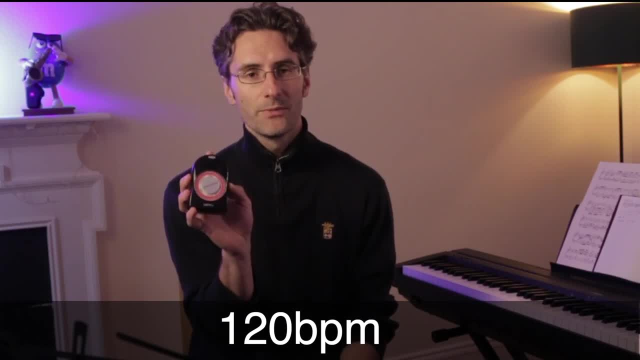 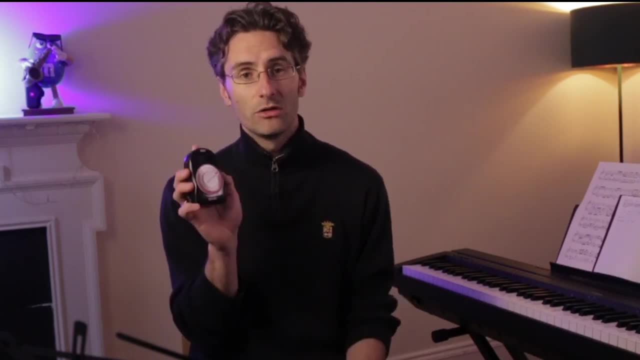 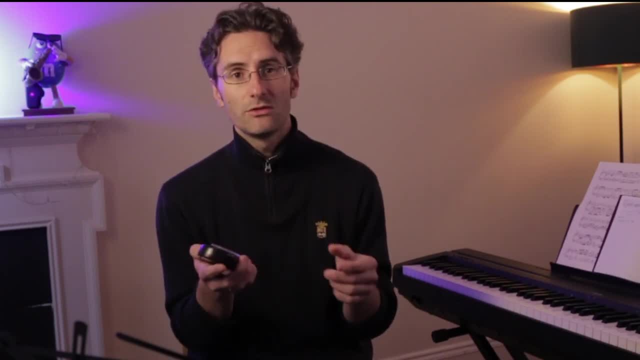 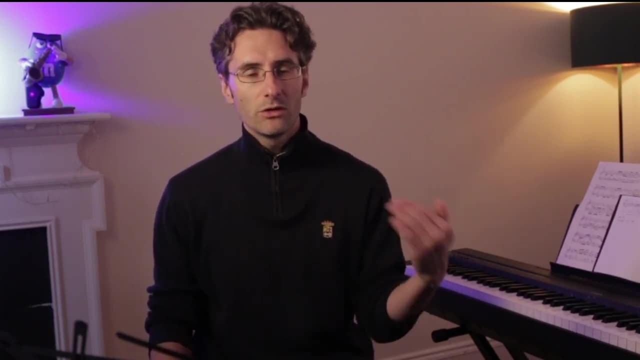 hands are always. my hand is always with the metronome in this case. so those are quarter notes. now eighth notes: do exactly what i do. okay, just copy exactly what i do. so we're going back to playing our quarter notes. okay, no metronome for now. you just play your quarter notes. now have your. 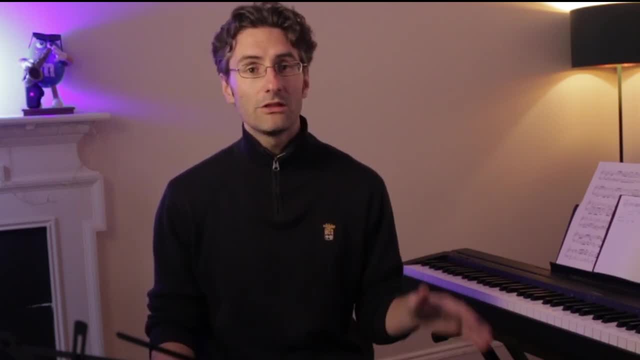 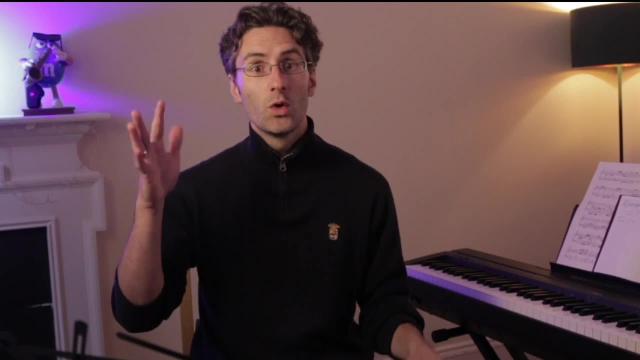 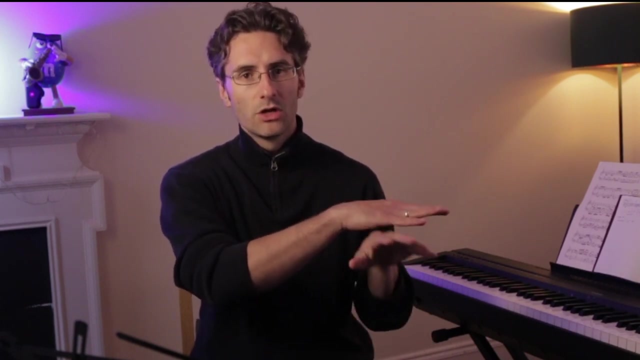 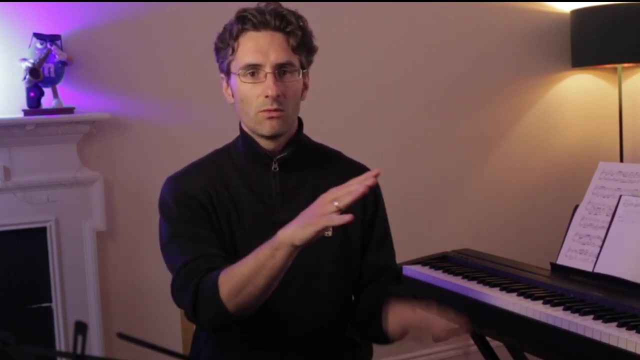 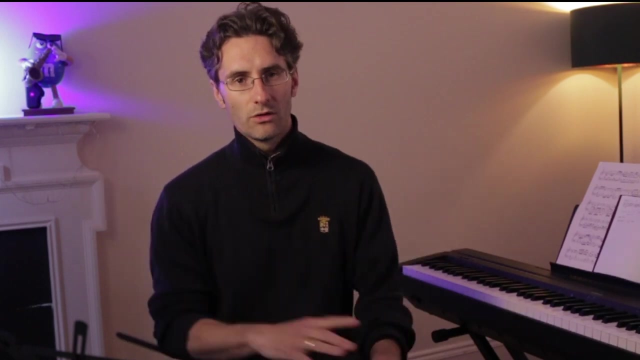 hand ready here with you, okay, and let's say the numbers. so one two, three, four again. one two, three, four, hand. one, two, three, four again. one two, three, four, no hand. one two, three, four. put it back. one two, three, four, no hand. one two, three, four, okay, so what's happening is, by the way, you can do this without the saxophone, actually. 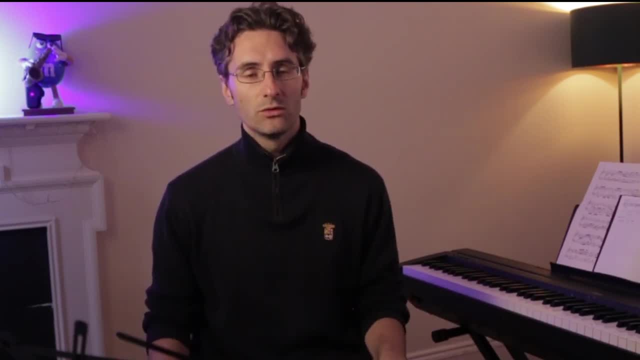 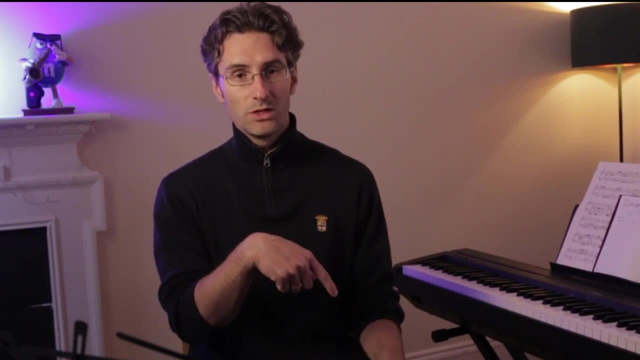 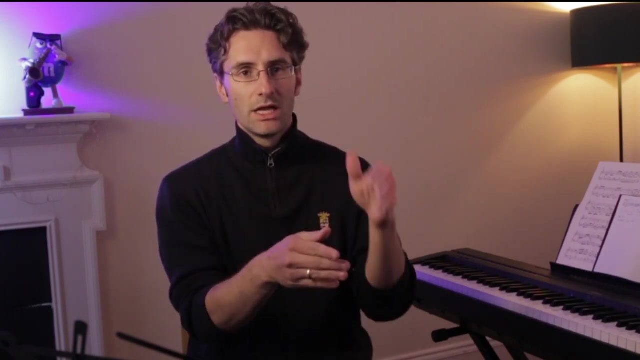 you should do it without the saxophone. that's way better way to to get everything, to ingrain everything in your brain. so what's happening? this is the quarter note. okay, we know that when i put my hand on top, what happens is i basically divide the beat into two equal parts: one and two and three. 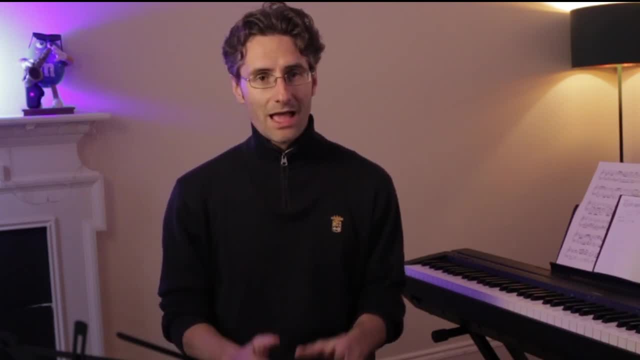 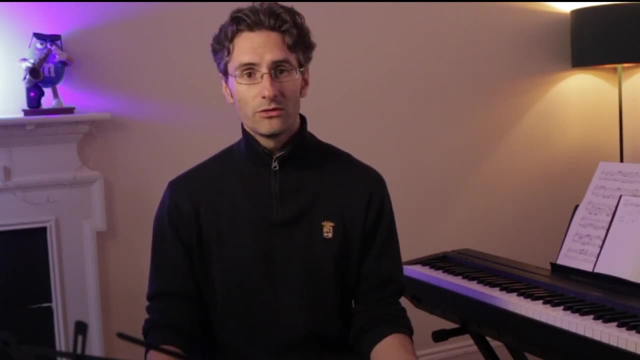 and four and and so and so forth. okay, instead of using the traditional method of counting one and two and three and so on. um, something that i learned from drummers, and especially with benny grab when i went to study with him a while ago, is that drummers use words to ingrain the rhythm of 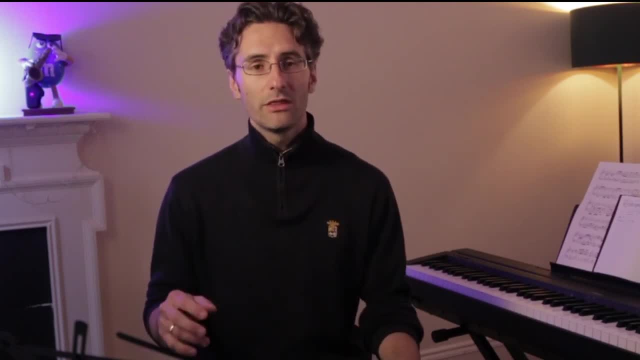 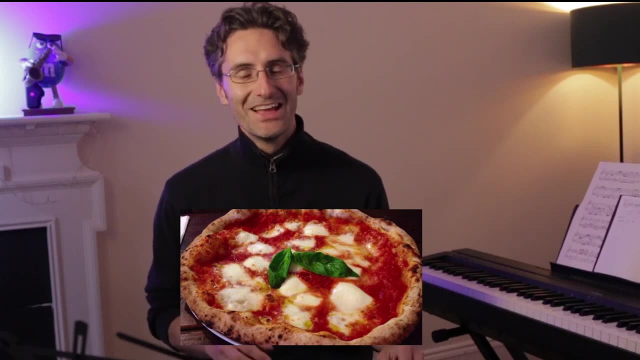 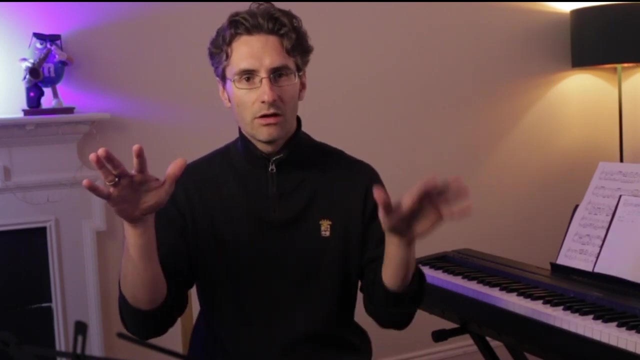 whatever they're doing, okay. so in this case, for simple eighth notes, you can think of any two syllable word, and i like to think of pizza because pizza is nice, so we can say p pizza, pizza, pizza, pizza, pizza, right? so, whether i have my hand on top or not, 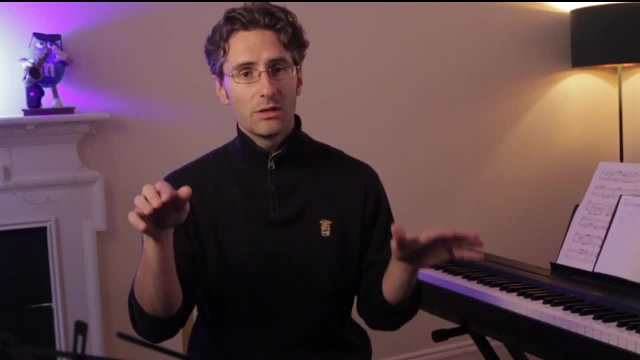 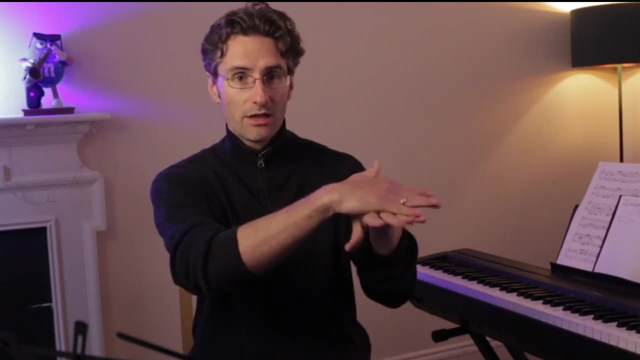 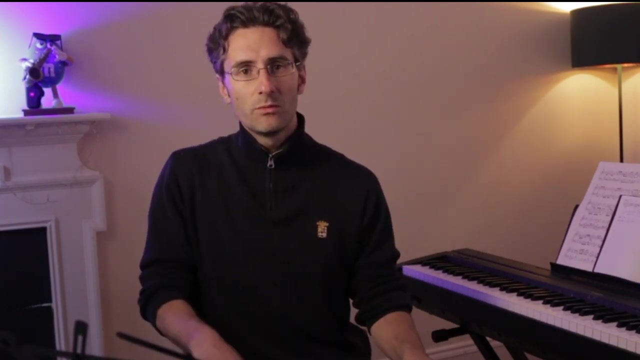 my pulse here. my quarter notes are always steady. and then when i put it back, pizza, pizza, pizza, pizza. when the p is down and the tsa is up here, okay, if we deal with the metronome, let's do it together. so that's a 60. let's do one bar of quarter notes and one bar of eighth notes ready, one, two. 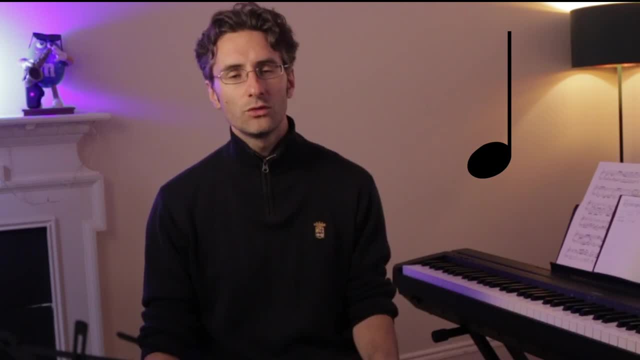 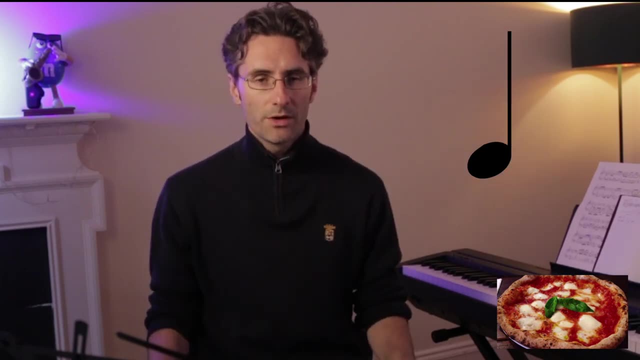 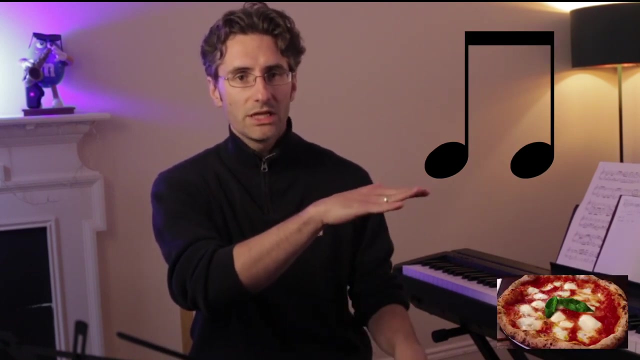 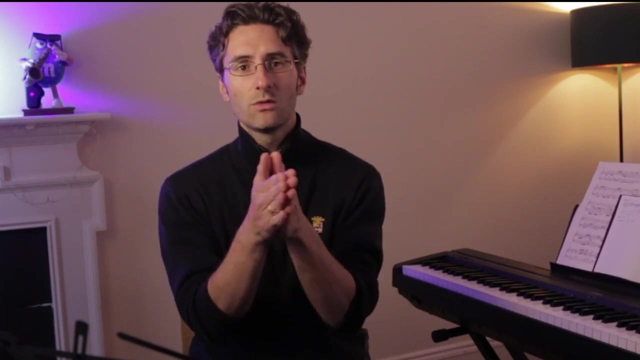 three and quarter notes: one, two, three, four. one two, three, four, one two, three pizzas, pizza, pizza, pizza, pizza. okay, makes sense, so that's a really great way to ingrain that in your brain. so anytime you see quarter notes on the page or you know that you're playing quarter notes by ear, just make sure. 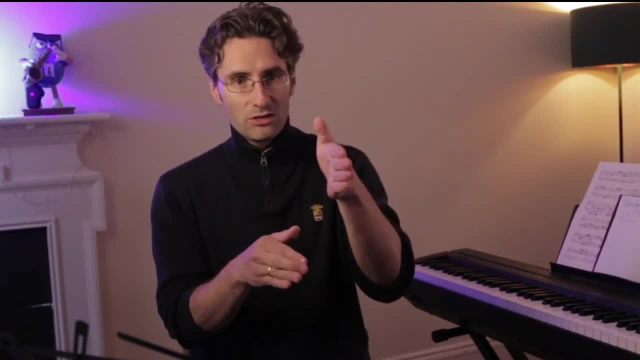 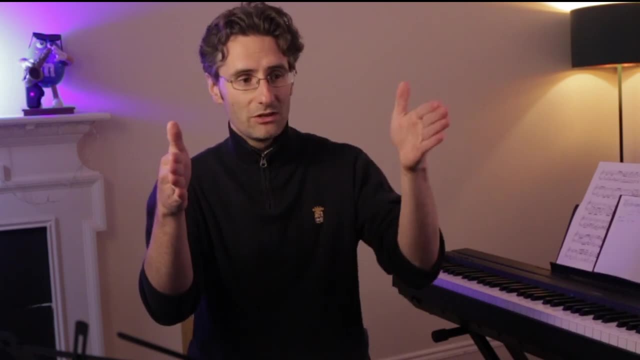 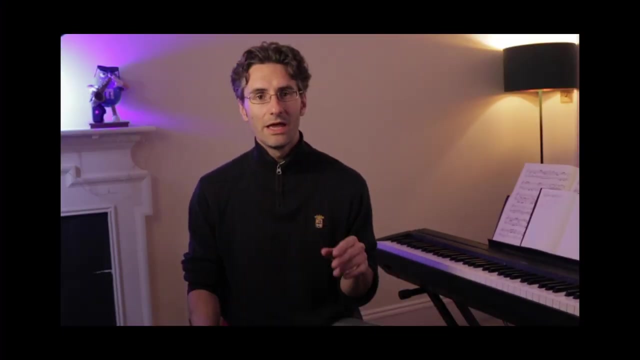 that they're equally divided. you know you have space between the beat and this beat and it's it's. what's most important is how you divide, how you subdivide the space between the two beats so everything is nicely equally spaced, make sense, cool. and, by the way, for those of you who are in london on june 19th, we're 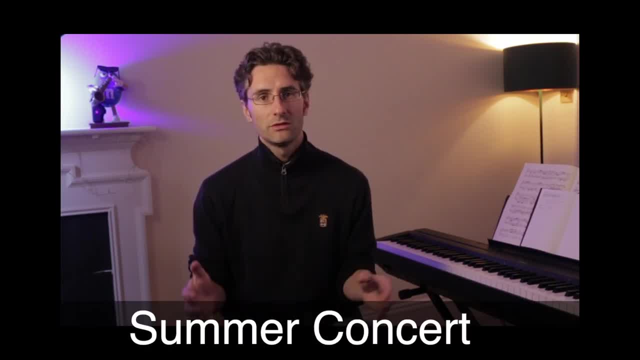 having an end of year summer concert. so if you want to come over, have a saxophone evening and just support our students, it'll be super, super cool to meet you and have you there. you can get your tickets here below in the description box and you can get your tickets here below in the 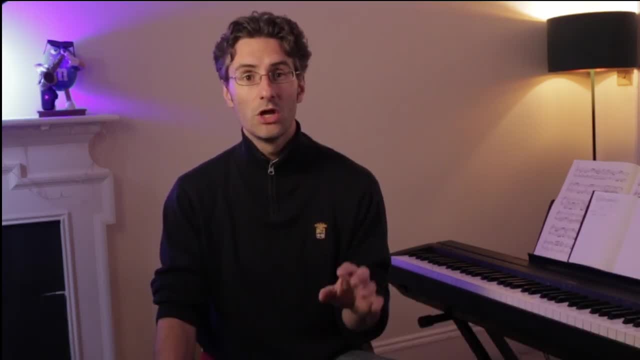 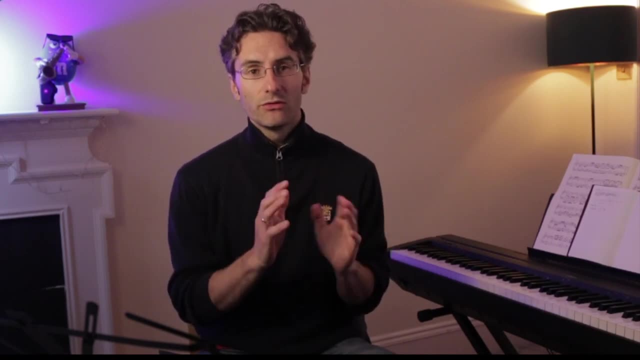 description, there's a link in which you can get your tickets. it'll be super awesome to have you there now. let's go into triplets now. the idea of triplets is no different from the idea of pizzas, of eighth notes. okay, what's happening is we have a beat and we have our next beat. okay, on pizzas, we. 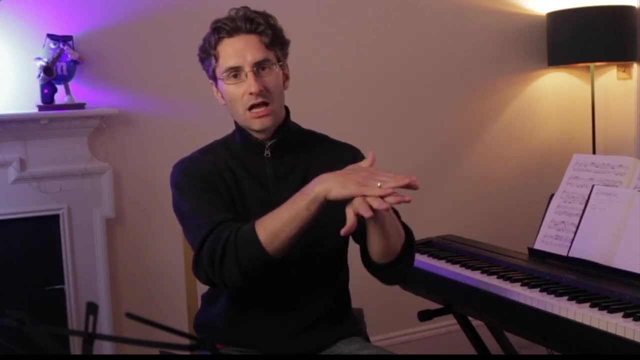 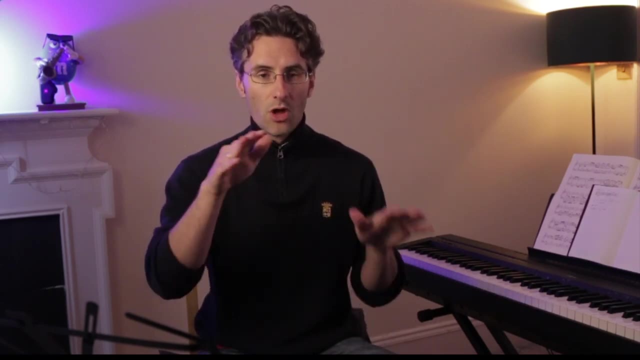 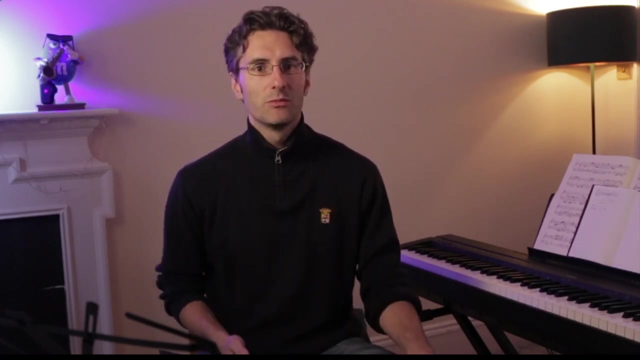 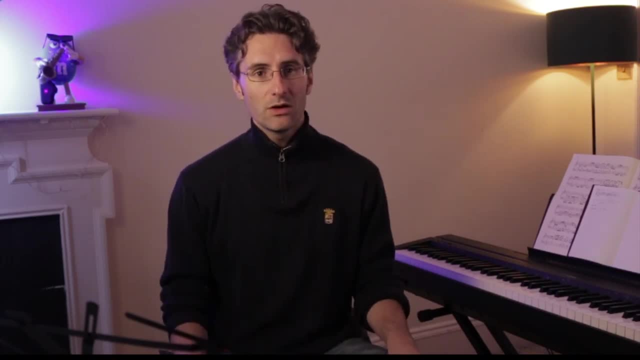 triplets. so we're just going to use another word instead, and that word is elephant, or any other three syllable word that you want, it doesn't really matter, okay for me, i just use elephant all the time in lessons. so elephant, elephant, that's what we want. okay, the idea on elephant. 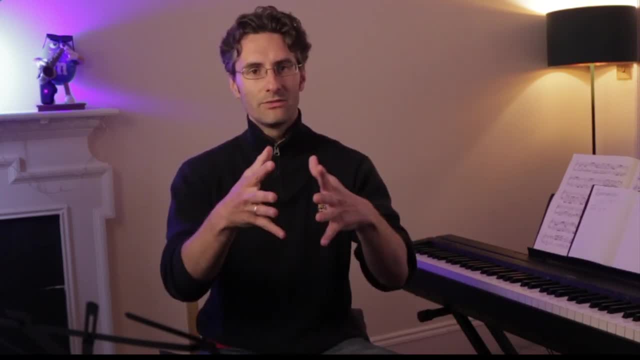 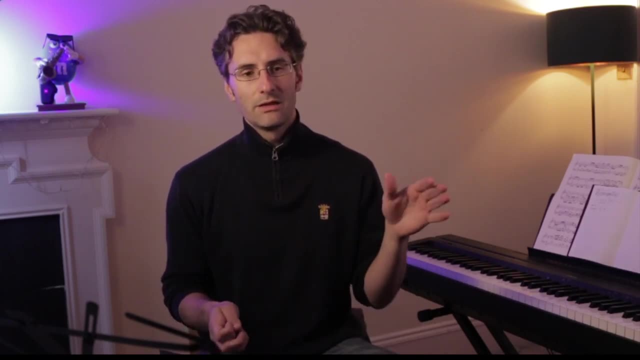 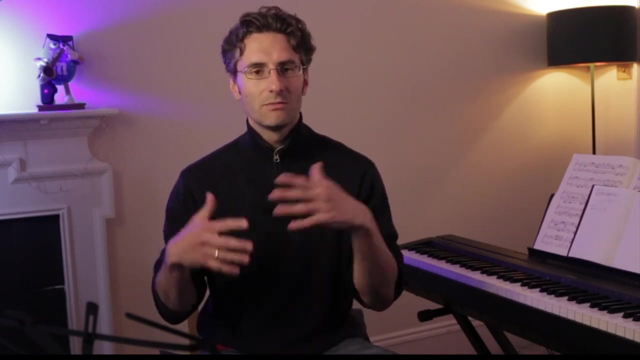 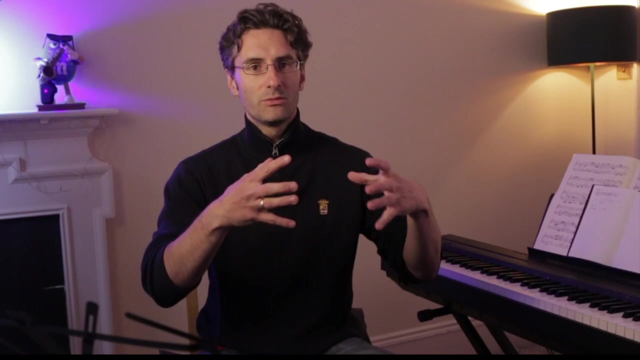 the idea on triplets is that you stretch that elephant so every single note is equally spaced between the two beats. okay, i see very often people saying things like elephant, elephant or like weird combinations, variations on the rhythm. so you want to be having, you want to have a very nice and equally spaced elephant, in a way. 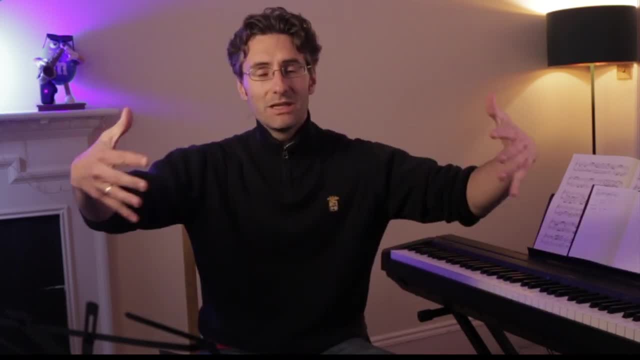 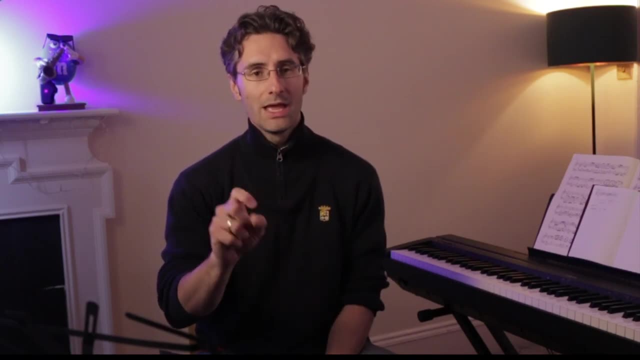 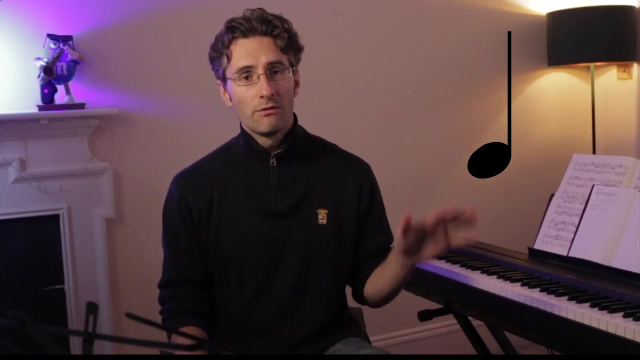 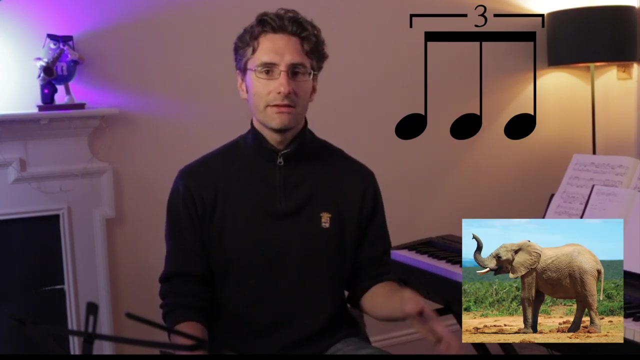 make it brief kind of thing, okay, so let's do it together. let's do one bar of quarter notes only and one bar of elephant only. okay, ready, without metronome: one, two, three and and four. one, two, three, four, elephants- quarter notes: two, three, four, elephants, elephant, elephant, elephant, elephant and so on. okay, the. 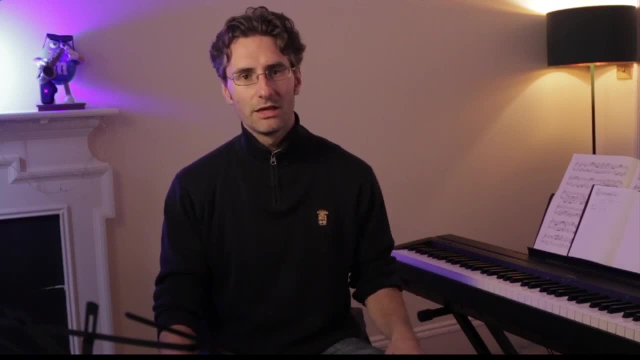 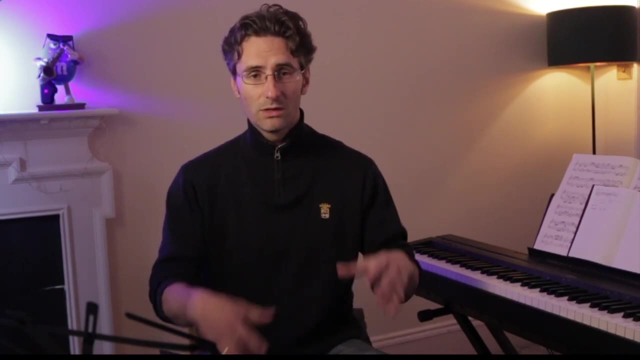 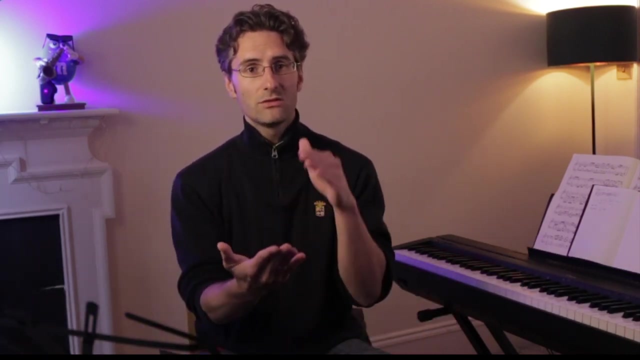 elephant has to be equally spaced, otherwise you get something like elephant, elephant, elephant, elephant, elephant, stuff like that. okay, which you don't really want. you want to have it nice and equally spaced, that's all it. that's, that's all. triplets are okay. if you think about triplets. anytime you see an, a triplet. 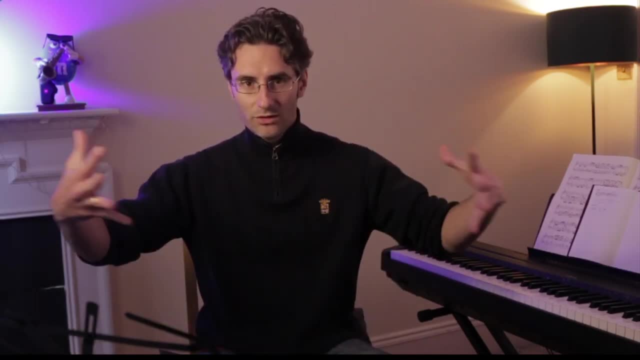 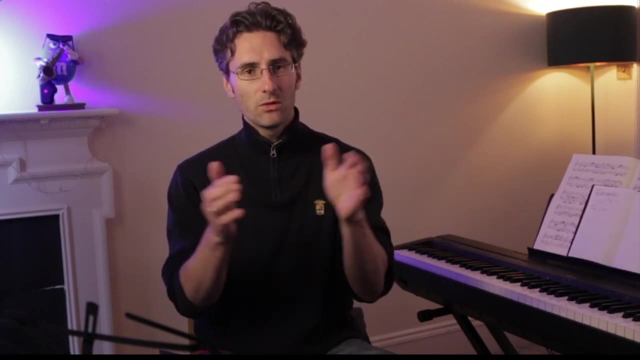 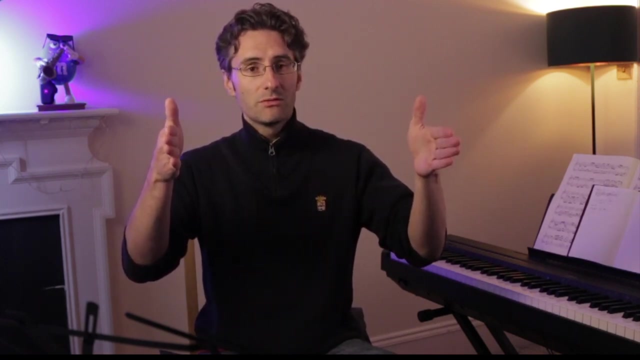 on the page. that's going to really save you. stretch it out, because that's the biggest thing. okay, and, and you'll be fine. now let's go into 16th notes. the idea is still the same. you want to divide, so Wait what I'm saying. you hide inside a single bar, very calm. so what you're going to do is you're just going to 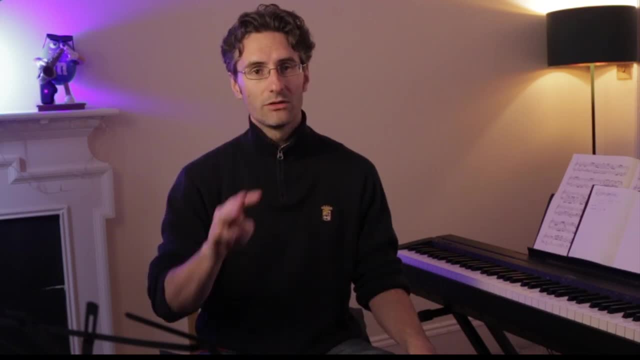 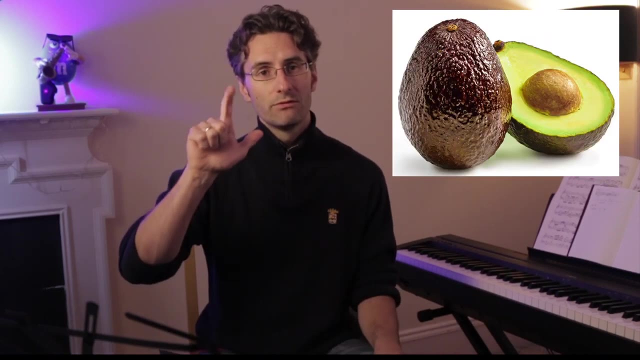 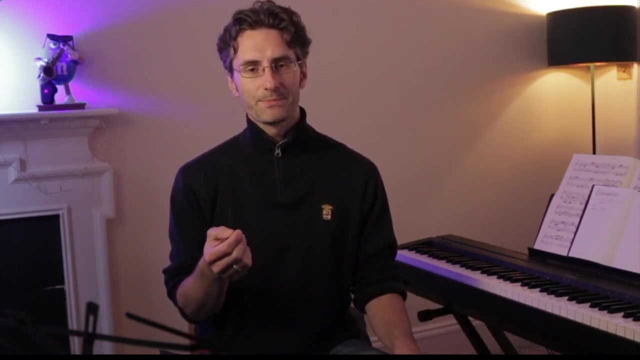 just going to bookmark your wrote, juxtapose one for the second or take out your container more you can immediately take out notes. so here's four parts, four beginning 10mar. two leaves we going to take out notes for you three body parts, two clothes, two balance sheets. 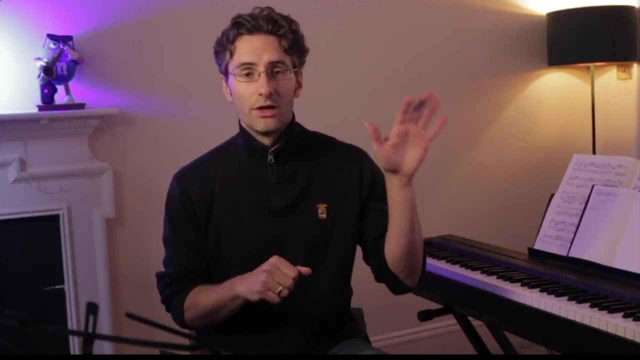 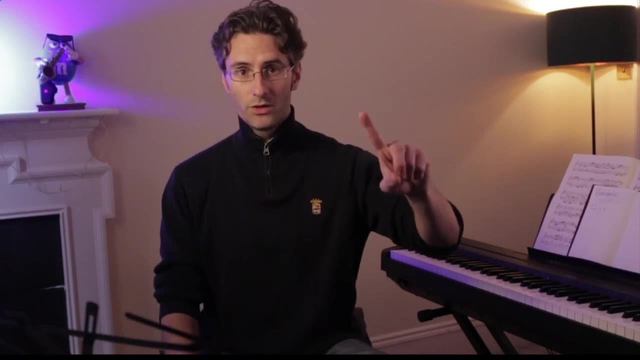 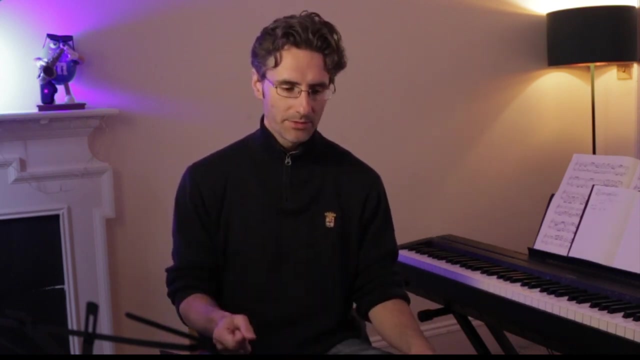 two other parts. So we're gonna go avocado, avocado, avocado, avocado Make sense. So let's do one bar of quarter notes to make it simple, to take it simple, And one bar of avocados Ready- One, two, three and four. 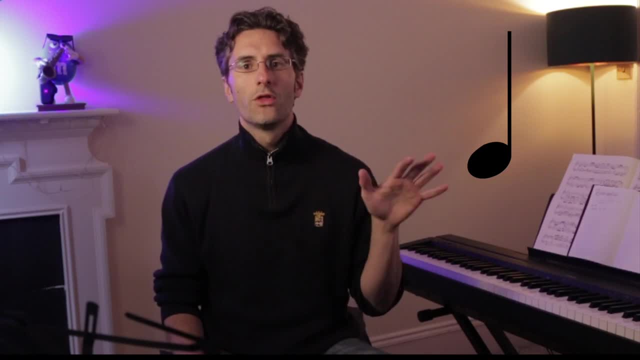 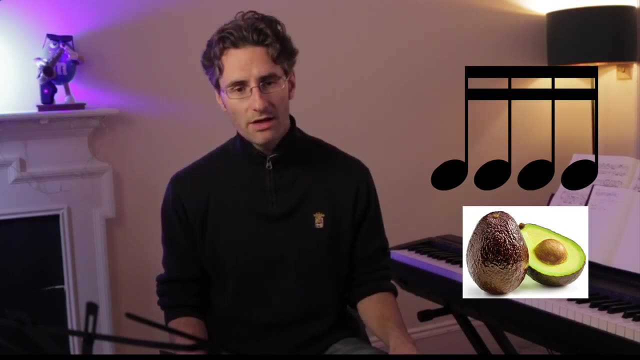 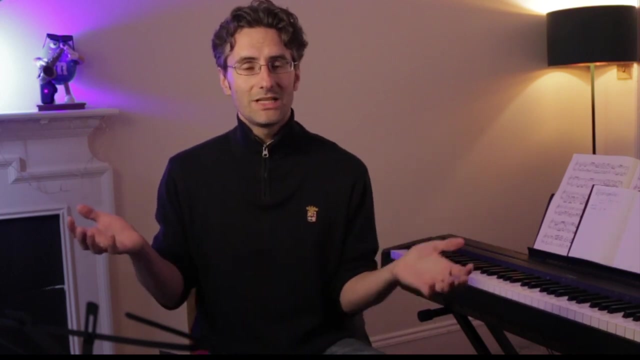 Here we go. One, two, three, four Quarter notes. Two, three, four, Again, Avocado, avocado, avocado, avocado. Okay, make sense. So that's all. that's all, it is okay. So 16 notes are basically just a bunch of avocados, make sense. 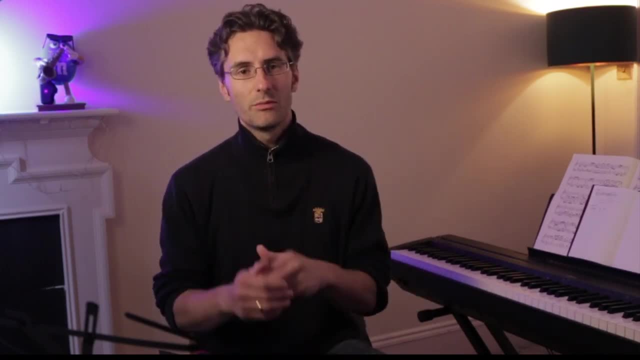 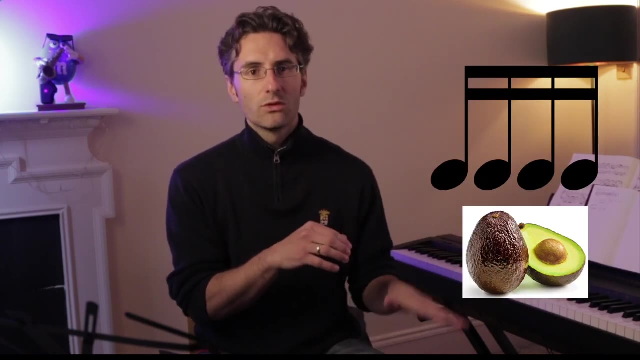 So, at the end of the day, we're relating everything to food apart from the elephants. So we have Pizza, Elephant, elephant, Avocado, avocado, And so on. okay, Make sense Now to put it all together. we're gonna do it this way. 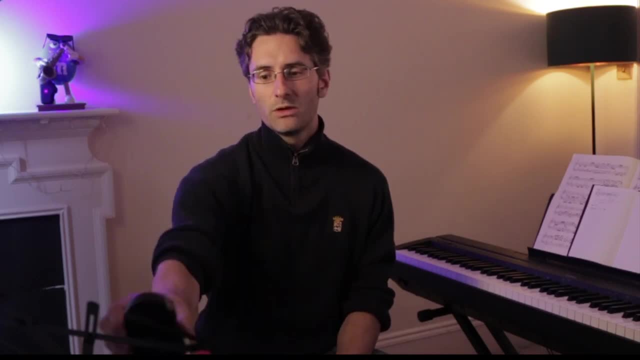 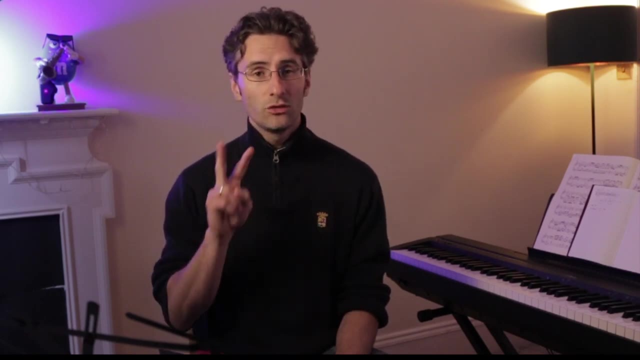 We're gonna take our metronome at 60 BPM, okay, And we're gonna do two bars of quarter notes, Two bars of eighth notes, two bars of pizzas, Two bars of triplets, two bars of elephants And two bars of avocados- 16 notes, okay. 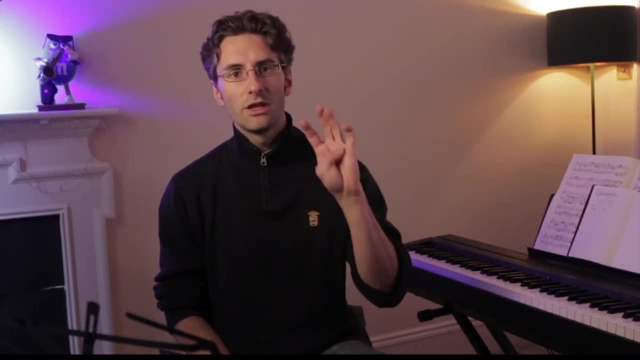 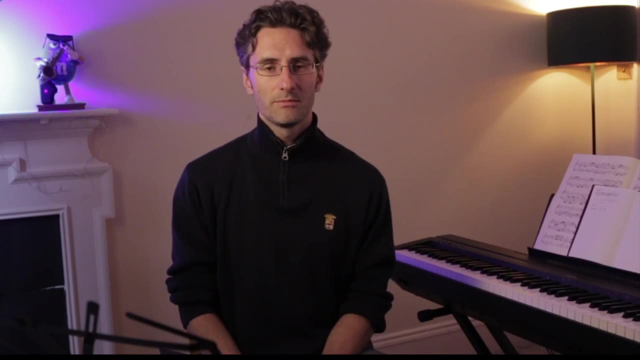 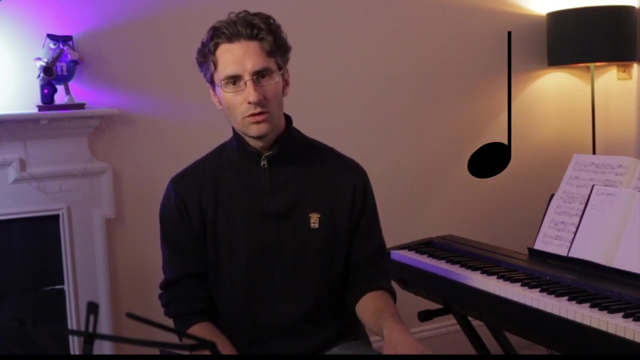 So Quarter notes: pizzas, elephants and avocados. Two bars each Ready, Here we go. That's metronome at 60. Here we go. One, two, three go. One, two, three, four. Again One, two, three pizzas. 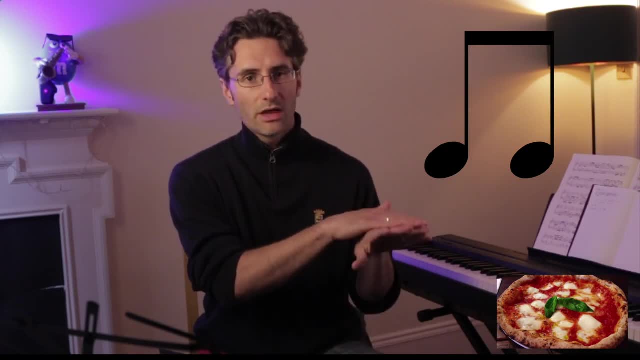 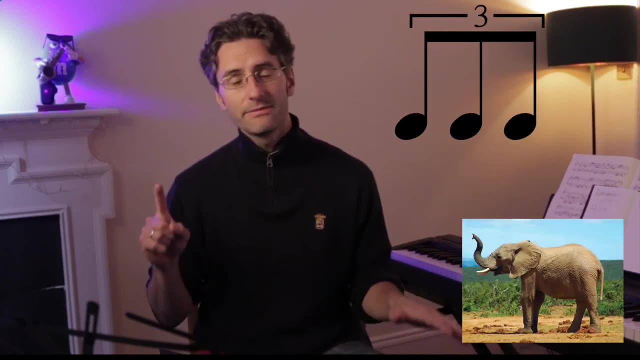 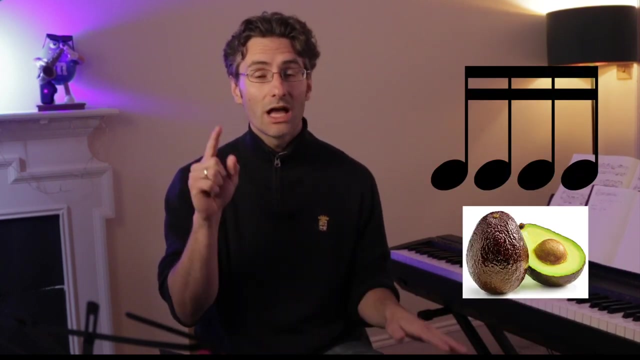 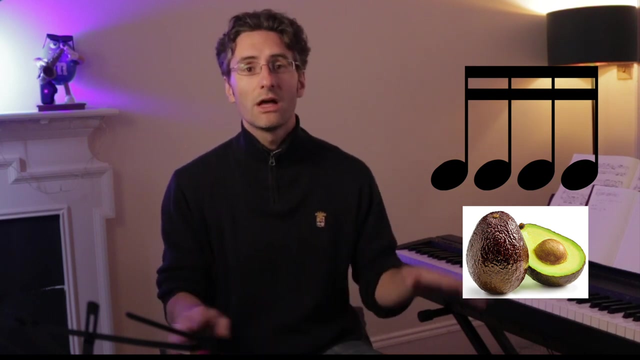 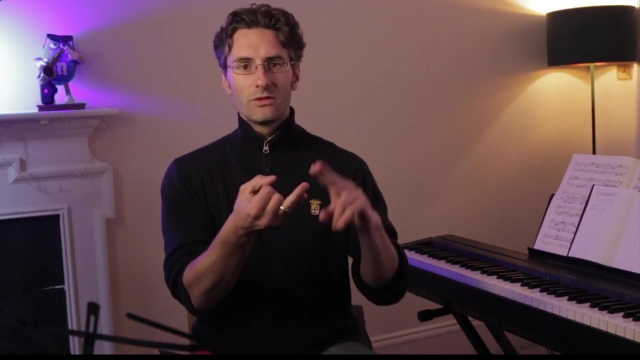 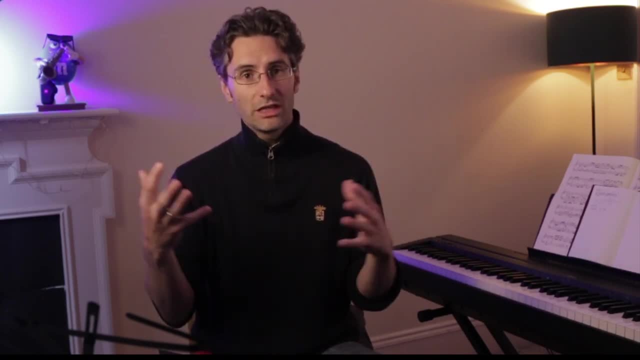 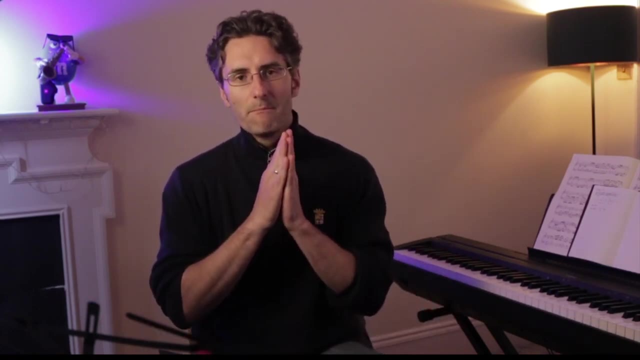 And you can relate to those And you can go back to thinking: Okay, those words, when you have the specific note values you know in in a piece of music, that's gonna be a massive game changer when it comes to playing into being more accurate rhythmically. okay, because